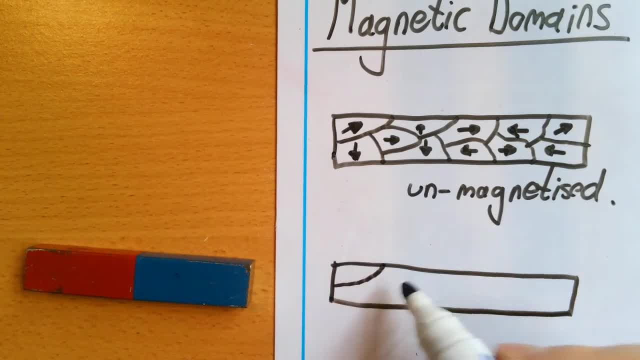 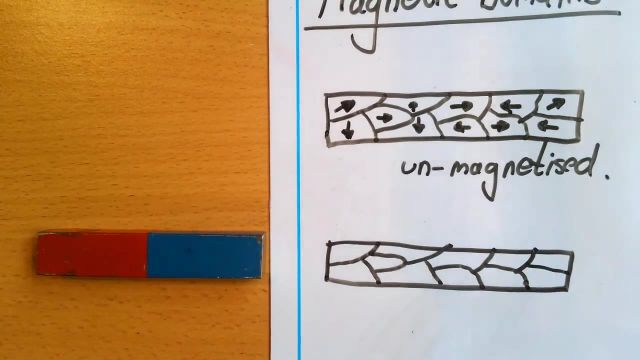 means is that the domains are in a very similar place, like that, but they're all lined up. Now this is where you would be careful on the direction, because the arrows inside point to north. so in this case, north is on the left, so all the arrows point to the left. So this is a magnetized bar magnet. so a magnetized 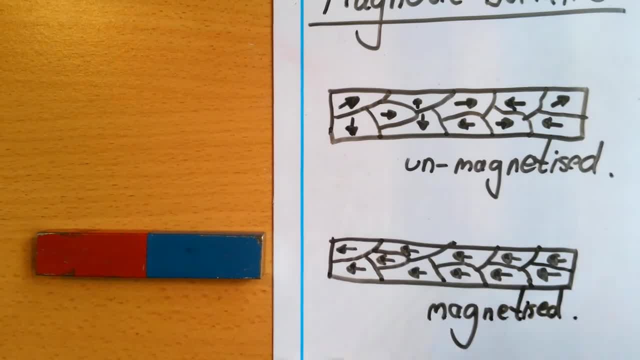 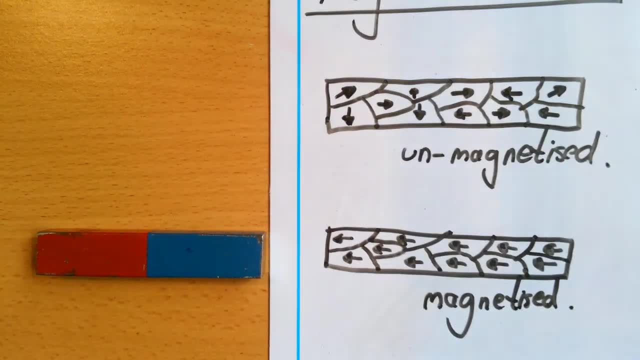 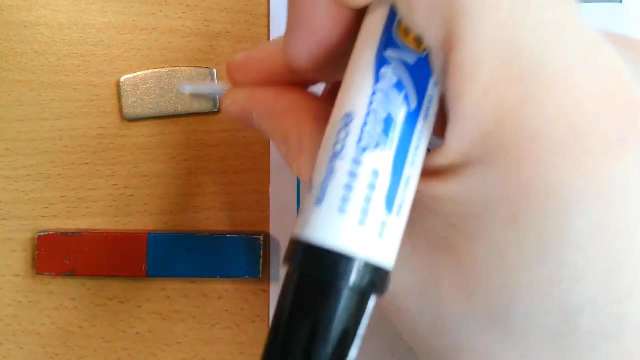 piece of iron, and if you've got your piece of iron in this shape, you call it a bar magnet, because it's just a bar, whereas something that is unmagnetized, like this piece of steel here that is currently unmagnetized, so we're bringing something else, that's magnetic material, near it. 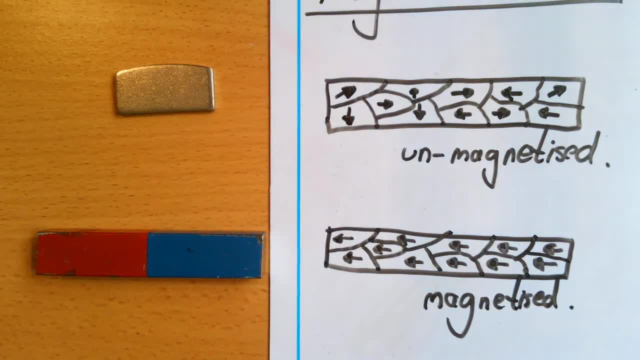 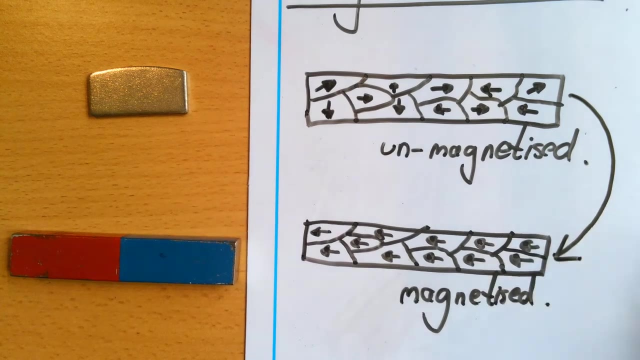 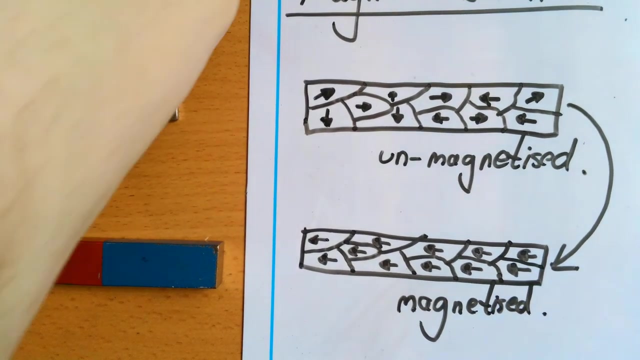 there's nothing, no forces, and so magnetic materials don't have to be magnetized. they can be unmagnetized. but there are ways to magnetize it, and if we were to represent magnetization in this diagram, getting from here to here is a little bit more being able to see everything. 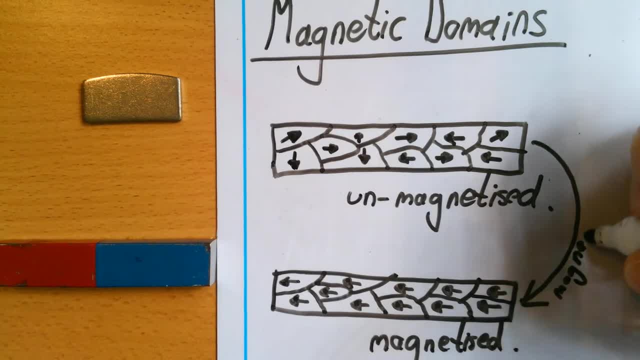 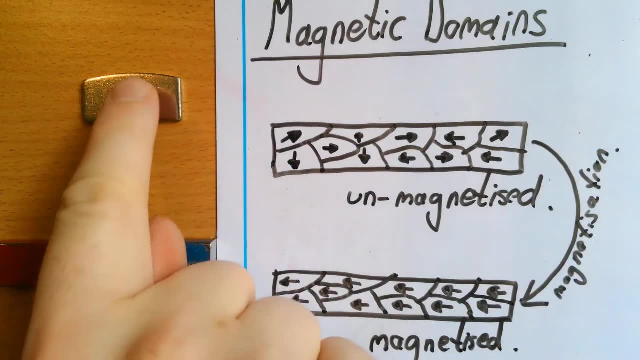 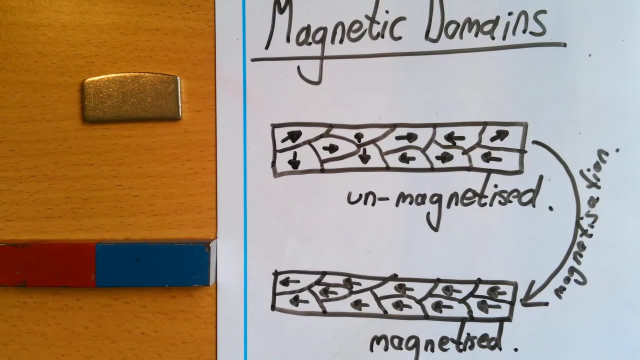 this is magnetization, sort of this in it. ok, so you take the unmagnetized magnetic material. when you magnetize it, the domains line up. that is what causes it to be magnetized. now in this video we're not going to particularly look at what makes up the domain and how the domains form. that's a 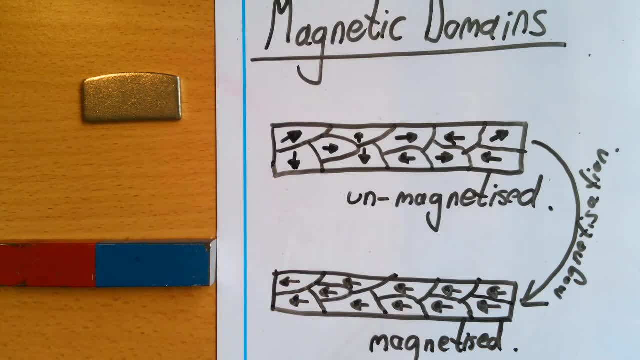 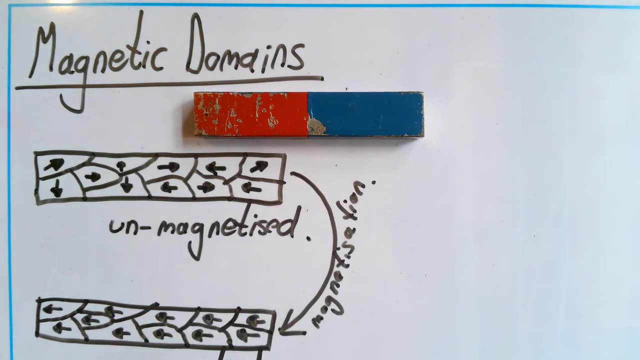 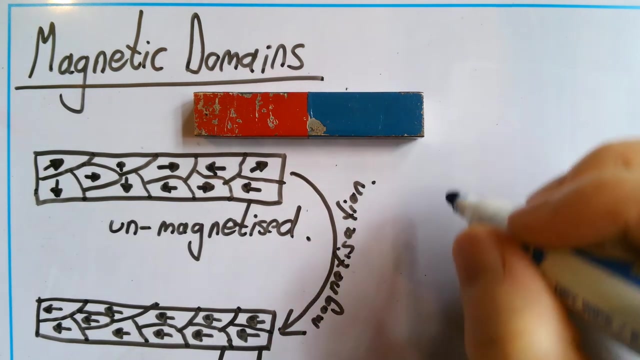 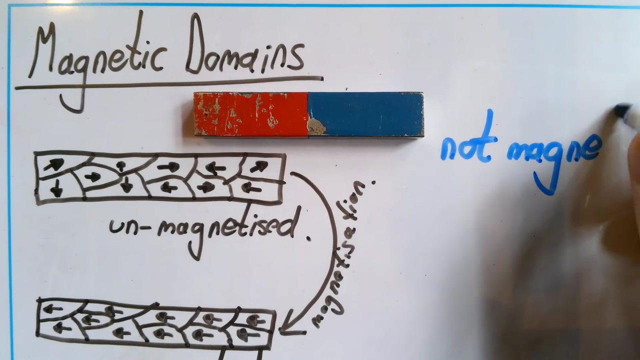 little bit more advanced. but as an explanation to why is a magnet magnetized, is because the domains within that material line up. What I'm going to do is put our bar magnet there for reference and in blue, so I'm going to say here: not magnetized as domains not lined up.